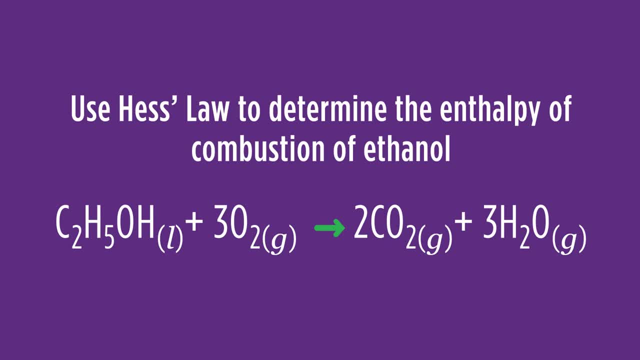 Here we have ethanol reacting with oxygen to give us carbon dioxide and water. To figure this out, we're going to need standard heats of formation for reactions that we can add up to come up with this actual chemical reaction. To do that, we'll need to find some Now, when you start off. 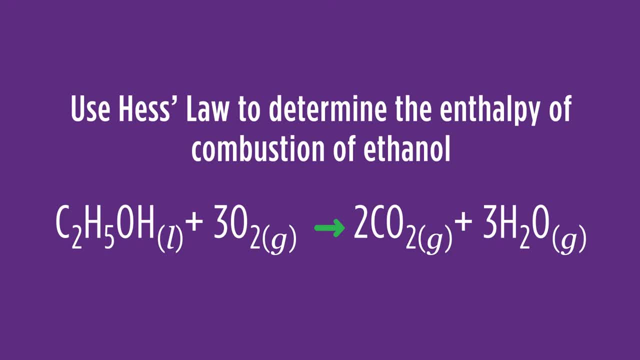 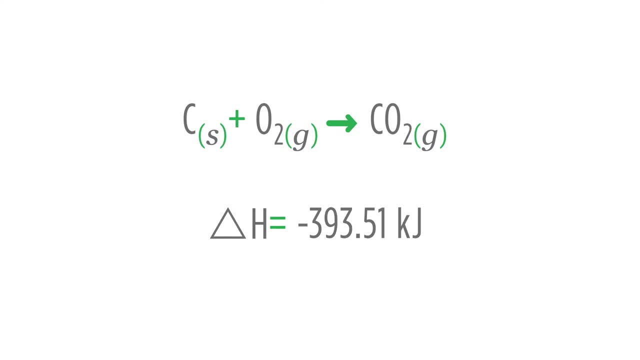 these will probably be provided, but you can also find these often in tables. Here are the three we're going to look at: Carbon plus oxygen going to carbon dioxide with a delta H of minus 393.51 kilojoules. Oxygen plus hydrogen going to water, with a 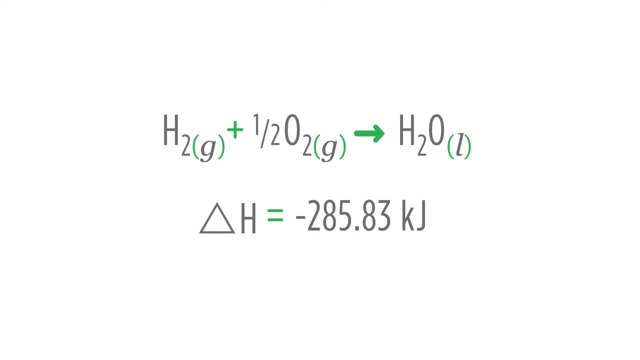 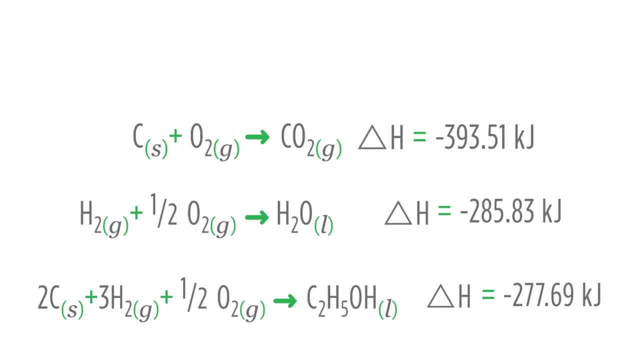 enthalpy of minus 285.83 kilojoules, And carbon hydrogen and oxygen going to form ethanol with an enthalpy of negative 277.69 kilojoules. What we need to do is take these three reactions and modify them so that it will give us the original reaction from the problem. 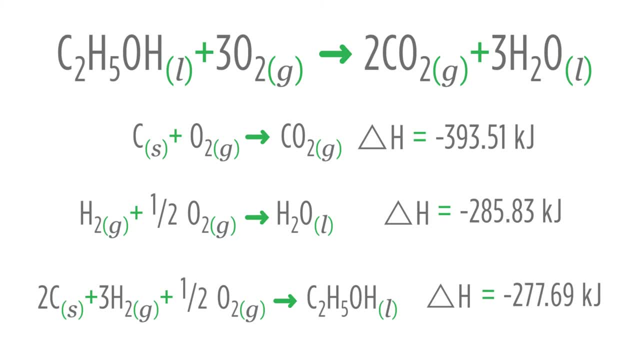 the combustion of ethanol. So we'll look On the product side. in the combustion of ethanol we see two carbon dioxides. If we look at our three reactions here, we see carbon dioxide is in our first reaction. But we had 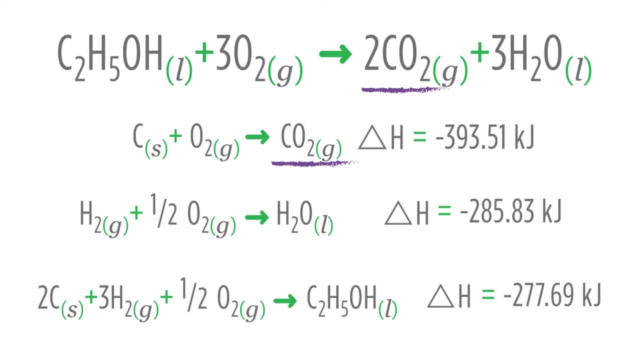 two carbon dioxides, which means we're going to take and multiply the entire reaction and the enthalpy by two. This will give us two carbon dioxides so that we can match our original reaction. If we look at our second, we have liquid water. Well, we had liquid water in the combustion. 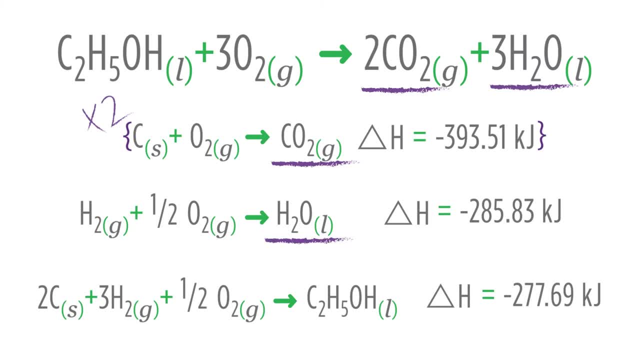 of ethanol, but we had three. So since we only have one here, we're going to need to multiply the entire reaction. So we're going to need to multiply the entire reaction. So we're going to need to multiply the entire reaction by three, including the enthalpy. Now, those were the 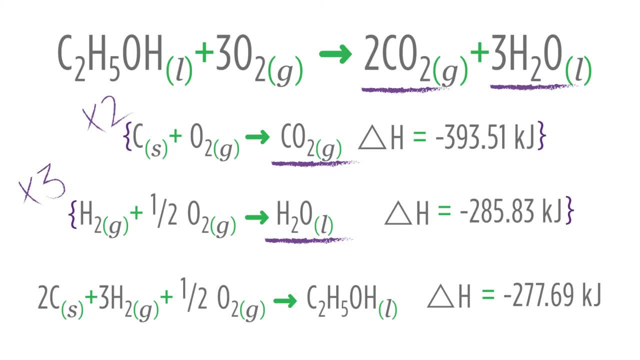 products that we had in our original reaction. If we look at our third, we have ethanol, But the problem here is that ethanol is a product, but we want ethanol to be a reactant. So therefore, we're going to have to reverse this reaction, which means that we're also going to have to 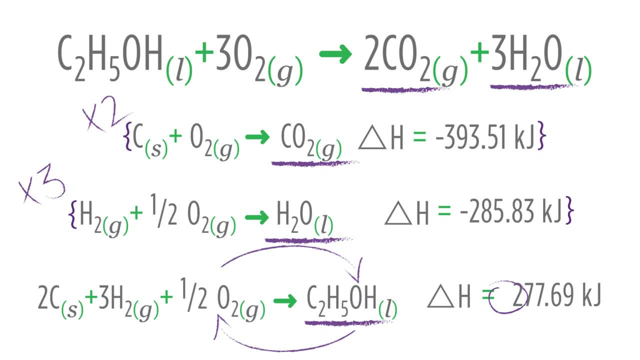 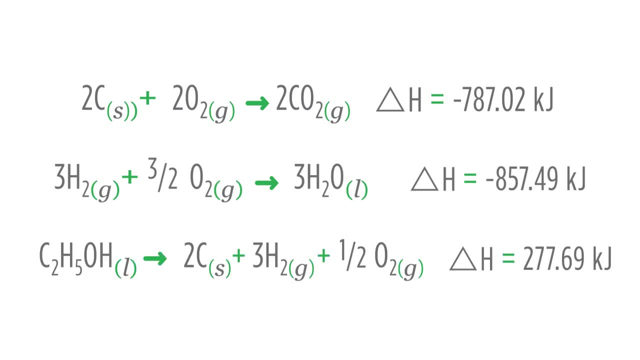 change the sign of our enthalpy. So let's do that. Let's multiply the first one by two, the second one by three and let's reverse The third and also make sure we change the sign. Now you can see that we have multiplied the first.